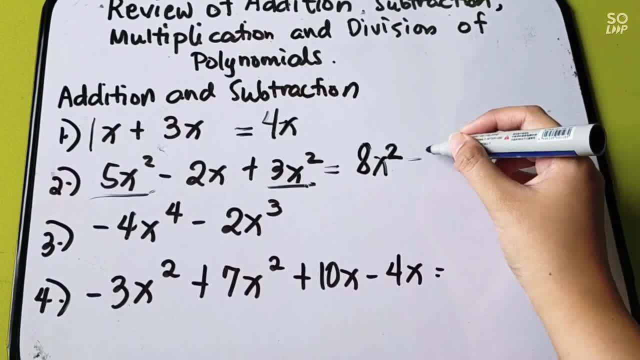 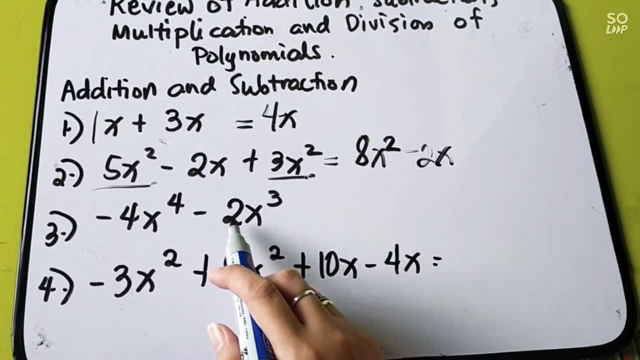 Then what you are going to do to negative 2x. you will just copy. So that's the answer. Is it clear? Next tayo, we have negative 4x raised to 4 minus 2x cubed. As you can see, we have different exponent here. 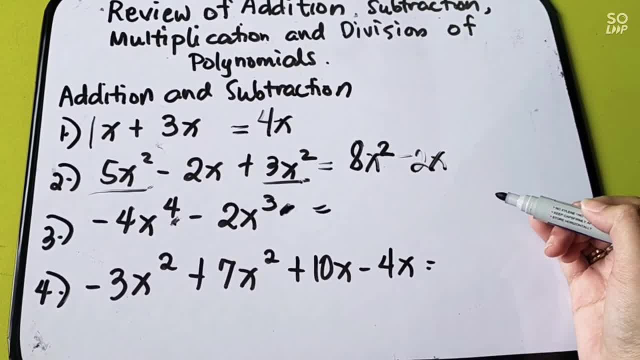 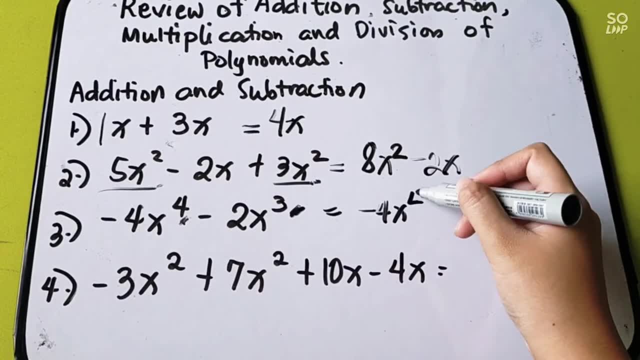 So kung meron tayong different exponent, no need to combine. Okay, We cannot combine them. So therefore the answer is negative: 4x raised to 4 minus 2x cubed. Okay, Next tayo we have here: 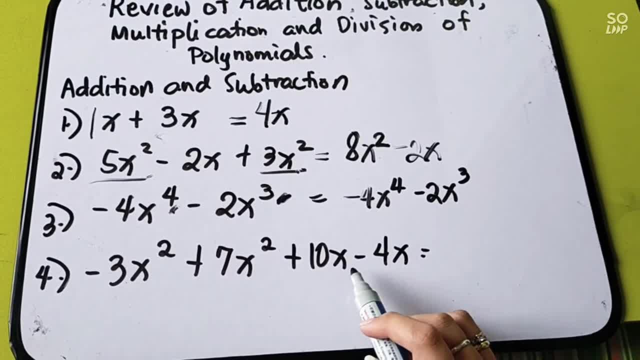 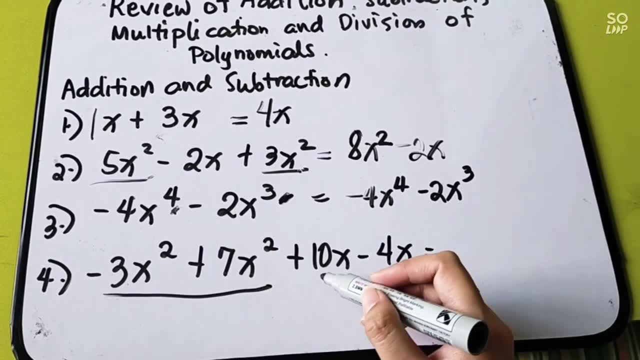 negative: 3x squared plus 7x squared plus 10x minus 4x. Hanap tayo na i-cocombine, So we can combine this two: kasa para sila na exponent and this two: Alright, So let us combine. 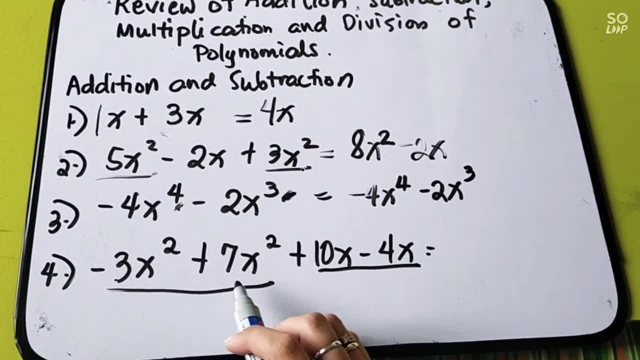 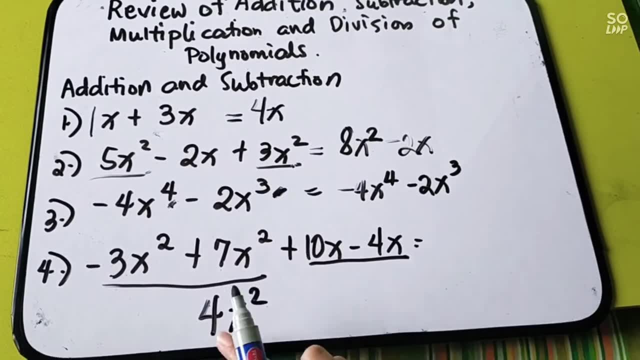 So negative 3 plus 7.. So negative sign you are going to subtract. So 7 minus 3, the answer is 4.. Just copy the variable 4x squared. Why positive Kasi mas mataas yung 7, which is positive. 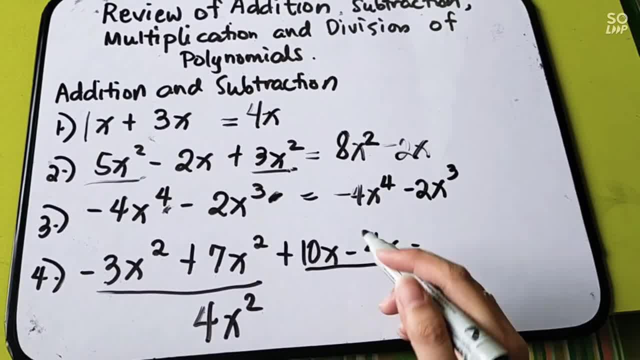 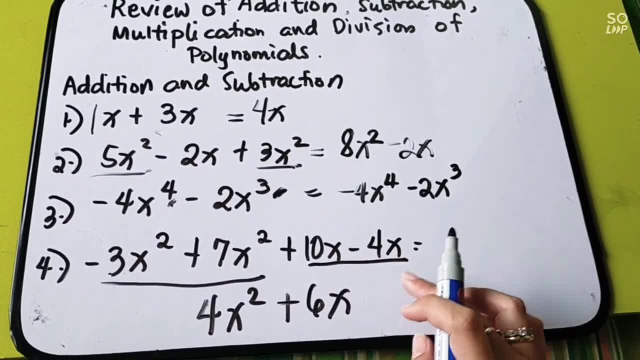 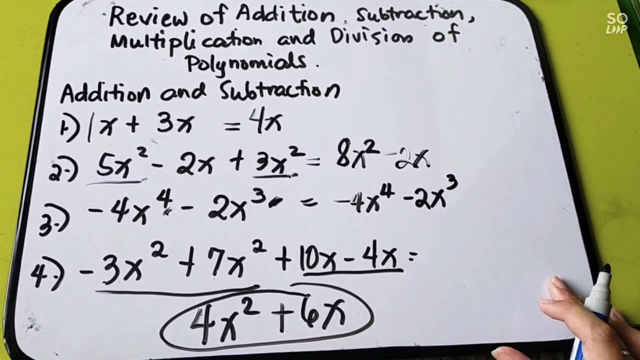 Alright. Next, 10 minus 4, the answer is positive: 6x. Okay, So just copy the variable. So this is your final answer. So that is addition and subtraction of polynomials. So you are going to combine like terms. 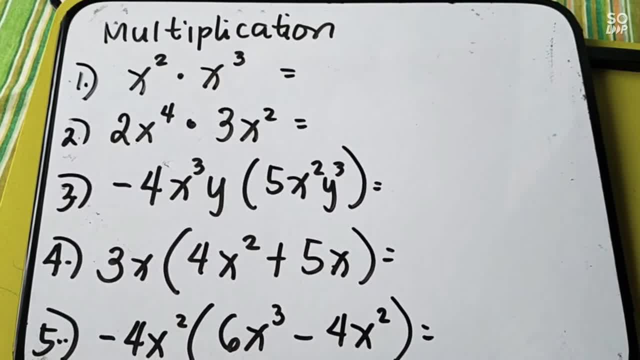 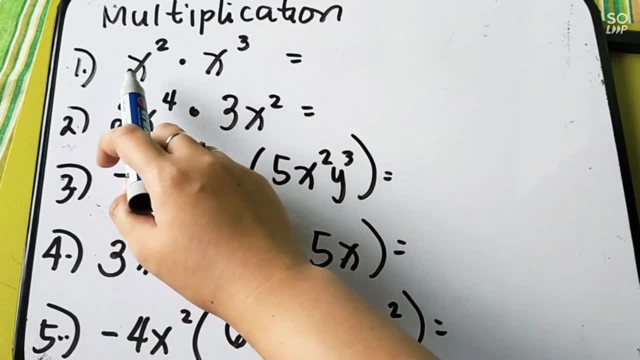 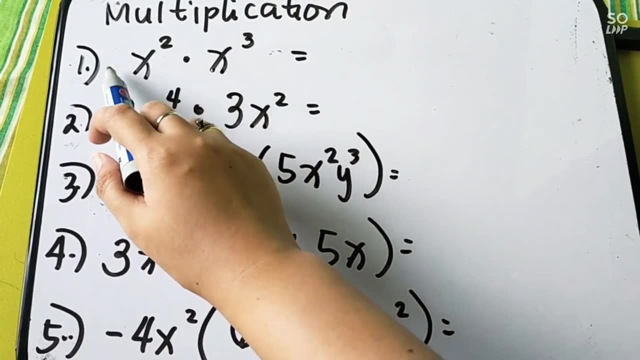 Let's move Multiplication. So let us multiply this one. If you have multiplication, this time you are just copy the variable, then add the exponent, The exponent ang i-add mo, Then yung numerical coefficient nya, yung katabi ng x na yan. 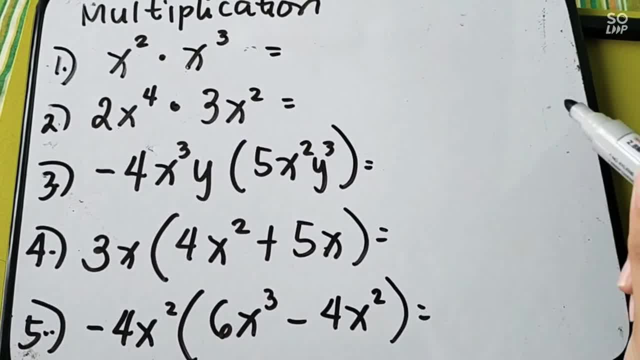 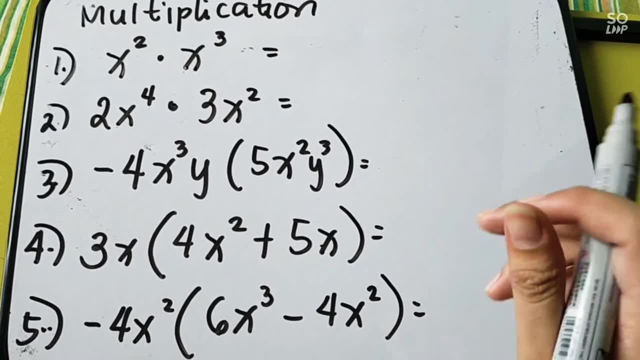 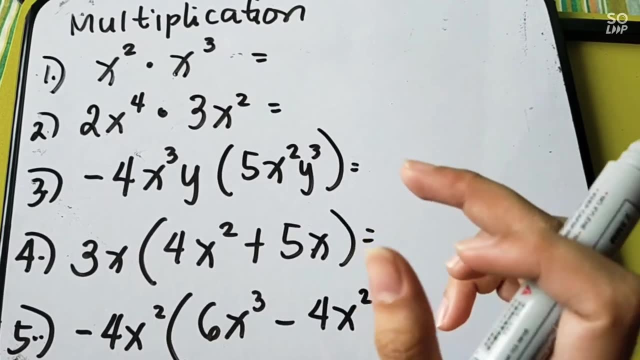 you are going to multiply, But the exponent you must be. add the exponent, Is it clear? So, kanina sa, addition and subtraction, you copy the variable and the exponent. This time, in multiplication, you copy the variable but you are going to add the exponent. 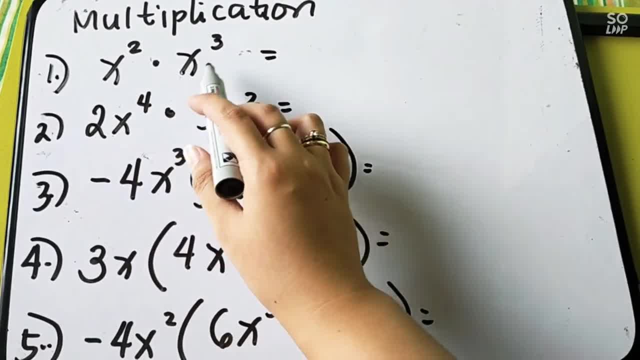 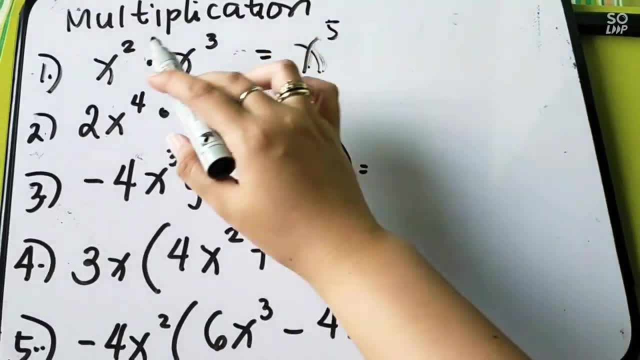 Is it clear? So we have x squared times, x cubed. So therefore ang sagot dito ay x raised to 5.. Just add 2 plus 3, we have 5.. Multiplication po ah. So next tayo. 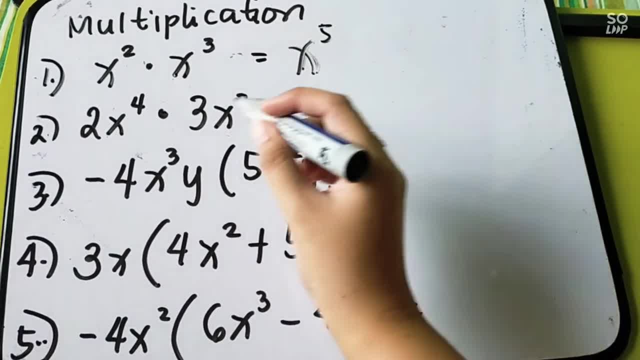 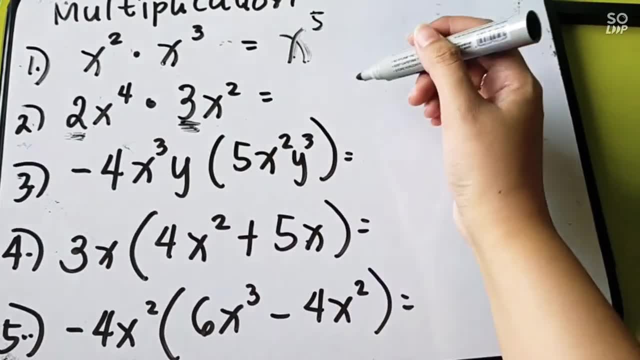 2x raised to 4 times 3x squared, Multiply the numerical variable, the numerical coefficient, Sorry, So we have 2 times 3.. The answer is 6.. Then copy the variable We have here, x, Then add the exponent. 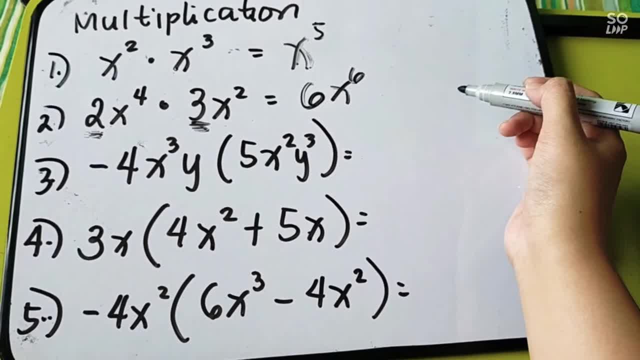 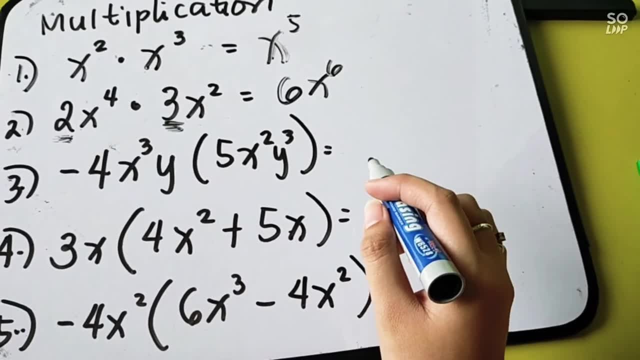 4 plus 2, we have 6.. So that's the answer. Next tayo This one May x and y. So therefore 2 variables are involved. We have x and y. Same process: Copy the variable, then add the exponent. 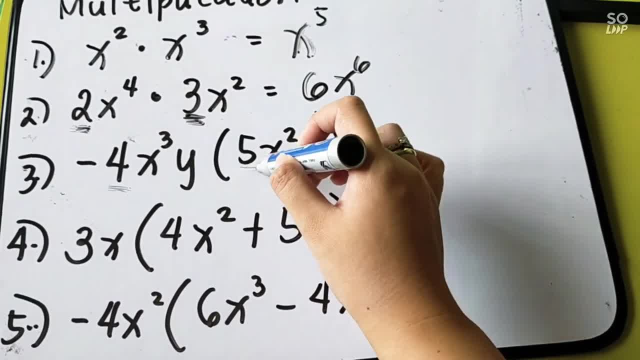 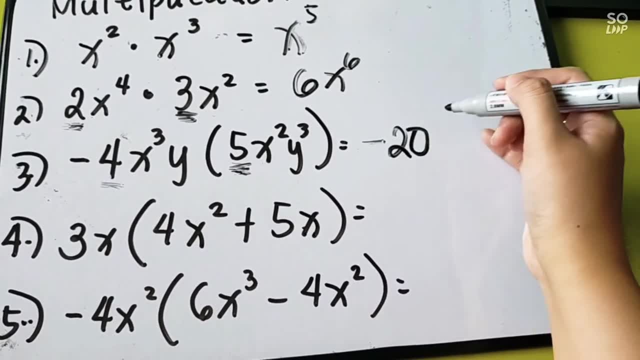 Multiply the numerical coefficient. O yan Multiply muna natin yan Negative 4 times 5.. The answer is negative, 20.. Then copy the variable x, then y, Then what's the exponent of x, 3 plus 2.. 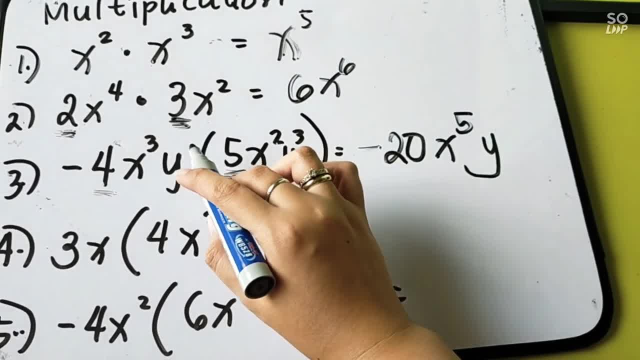 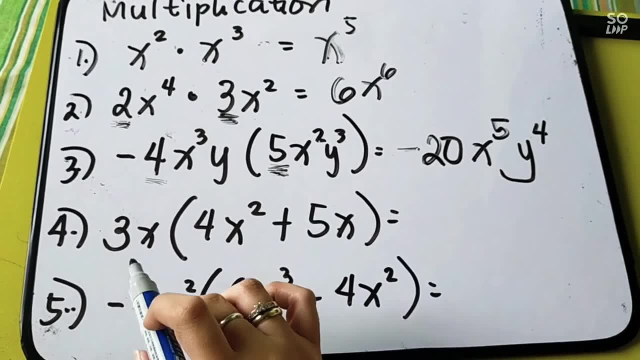 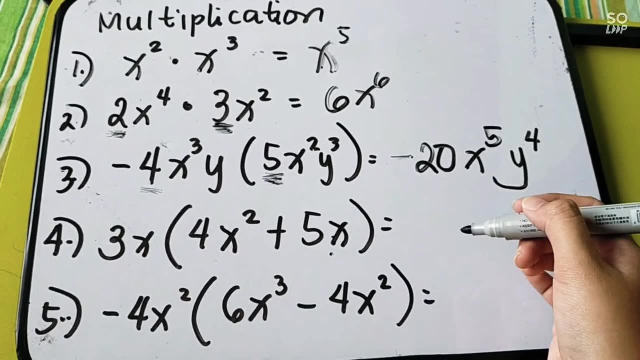 The answer is 5.. How about y 1 plus 3.. The answer is 4.. Is it clear? Next tayo, How about a monomial multiplied by a binomial? This time you are going to use a distributive property. 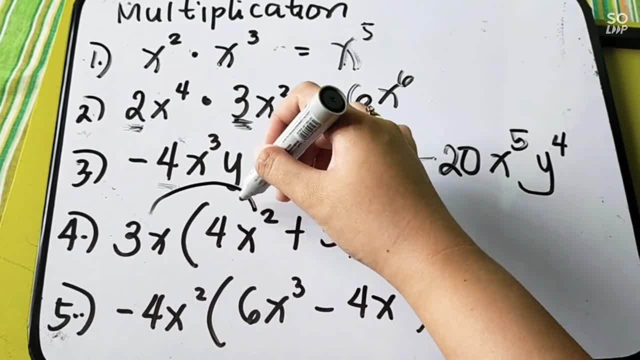 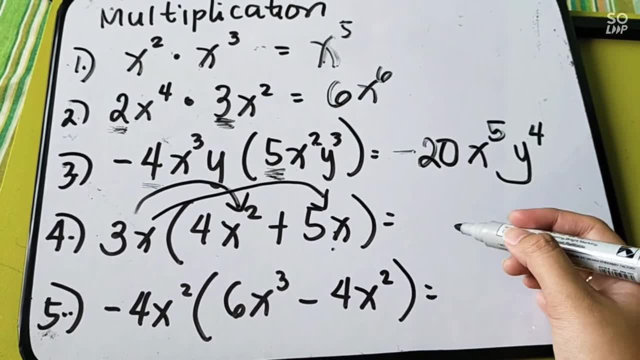 You are going to distribute 3x here. Multiply 3x to 4x squared, Then multiply 3x to 5x, Alright, So same process: Multiplication 3 times 4.. The answer here is 12.. 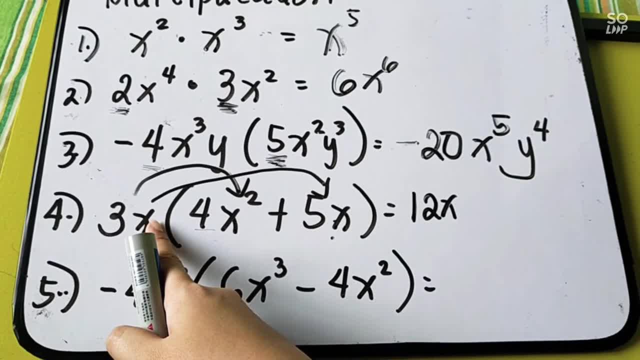 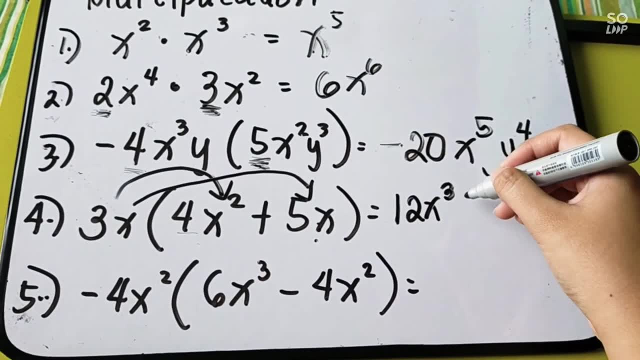 Then copy the variable. So this one, Ang exponent niya ay 1.. Dito ay 2.. 1 plus 2.. The answer here is 3.. Next Just copy the plus sign, Kasi binomial tayo. 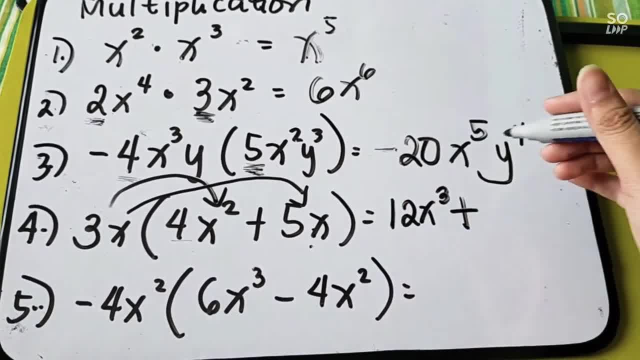 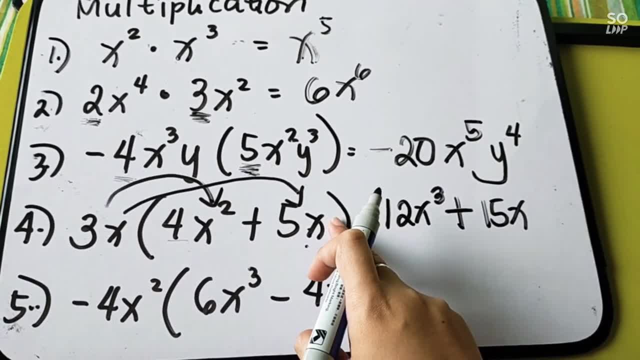 So yung 3 multiplied by 5. The answer here is 15.. Copy the variable again. We have here: the exponent is 1. Plus another exponent here is 1. 1 plus 1. The answer is 2.. 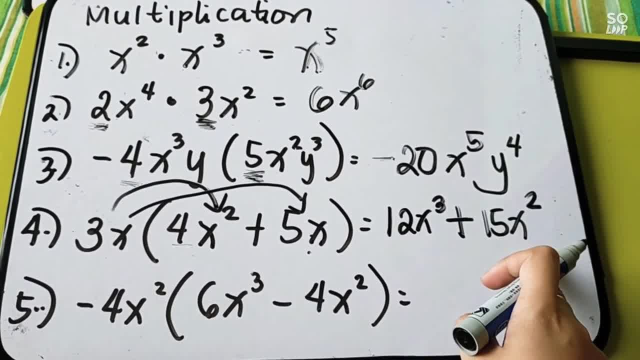 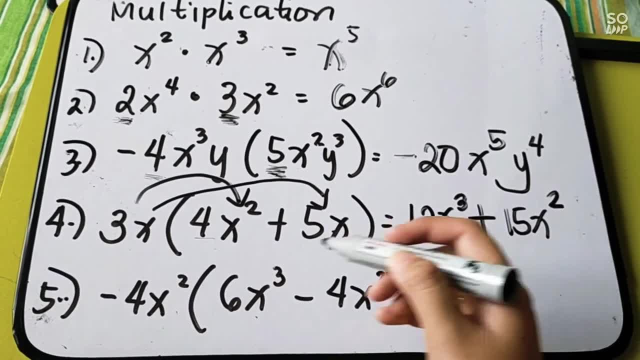 So the answer is 12x cubed plus 15x squared. Is it clear? Then, last tayo, We have negative 4x squared times: 6x cubed minus 4x squared. So same process, Multiply, Multiply. 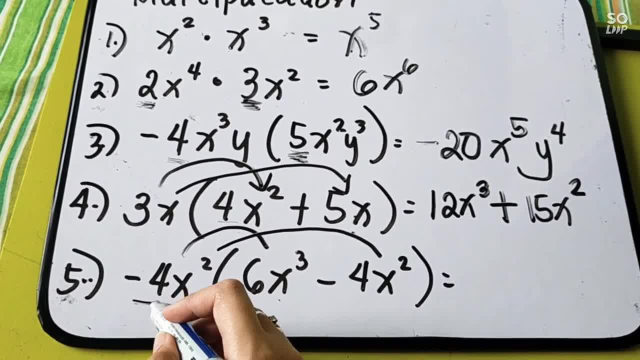 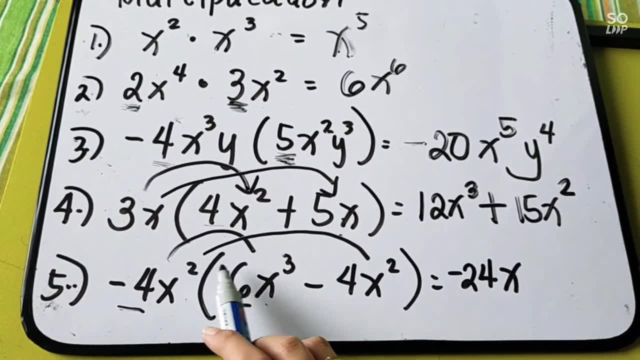 Distributive property. So we have negative 4 times 6. The answer is negative 24.. Copy the variable which is x, Then x squared times x cubed Add. We have here x raised to 5. Then distribute ulit. 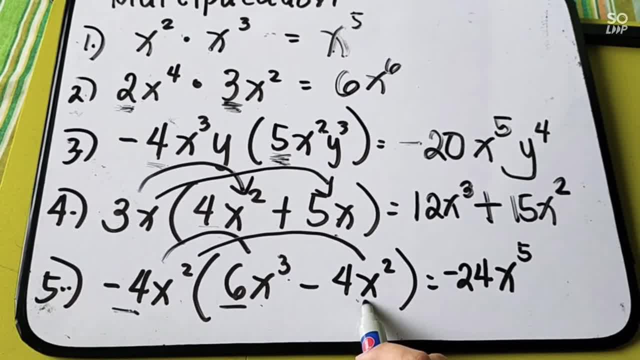 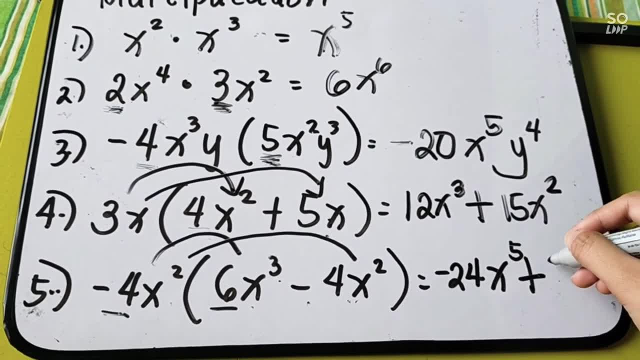 Negative: 4x squared times negative: 4x squared Same sila Diba. Negative times negative. The answer is positive, So 4 times 4.. The answer is 16.. Copy the variable x, Then add 2 plus 2 here. 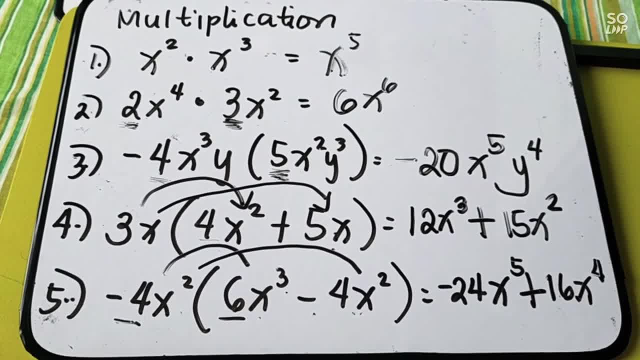 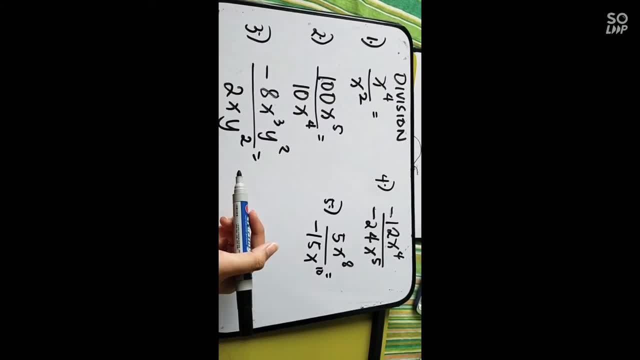 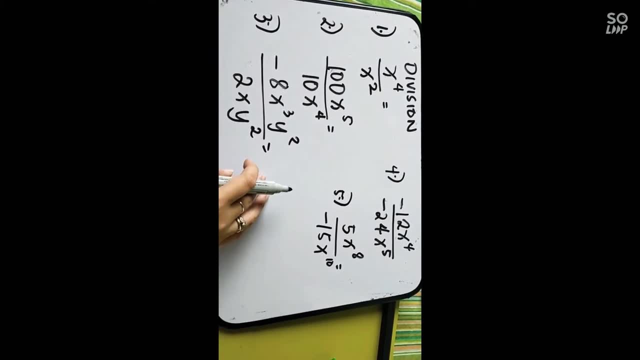 The answer is 4.. So that is how you multiply a polynomial. Let's move with division. Let's move with division. So we have here, If we have division, kabalik na rin naman sya ng multiplication, Diba kay multiplication, nag-a-add ka ng exponent. 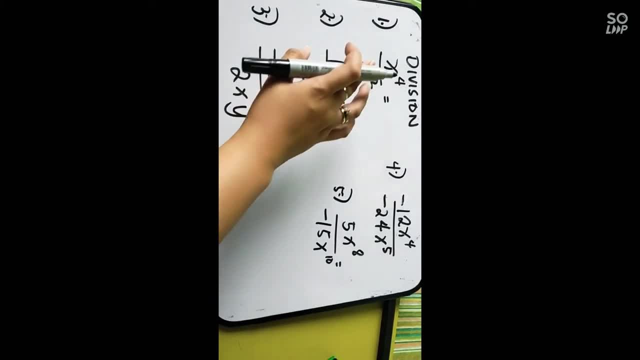 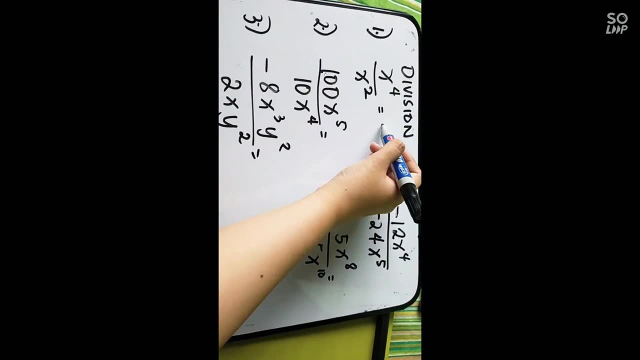 This time you are going to subtract the exponent. Copy the variable, then subtract the exponent. For example, x raised to 4 divided by x squared, Meaning x, x. So we have x here, Then 4 minus 2.. 4 minus 2.. 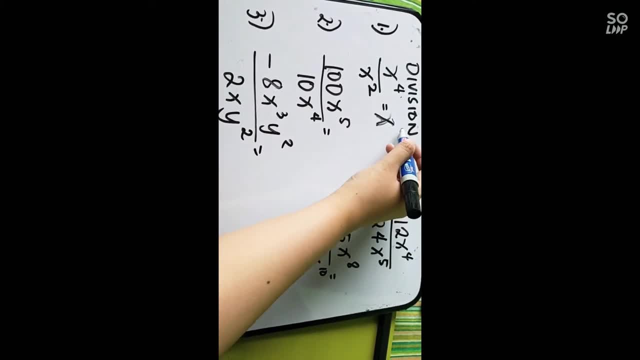 We have 2. So the answer here is x squared. That is it. Next tayo, If meron numerical coefficient, Ididivide mo si numerical coefficient, But kapag sa exponent You are going to subtract, Okay, So 100 divided by 10.. 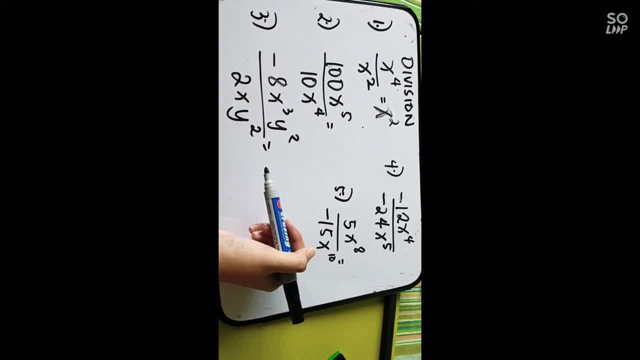 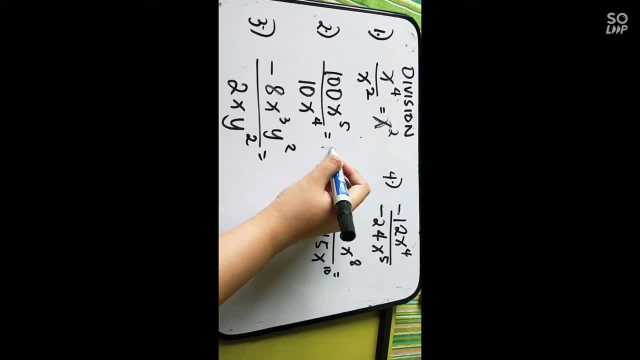 Ang sagot dyan, Ang sagot dyan, Ang sagot dyan. So plus 4 divided by 10.. Ang sagot dyan ay 10.. Ok-di-ba 100.. 100 divided by 10.. 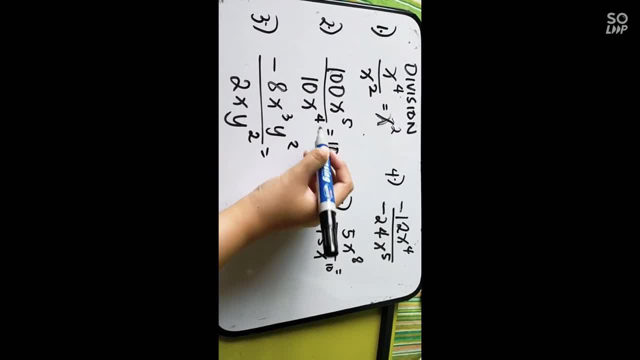 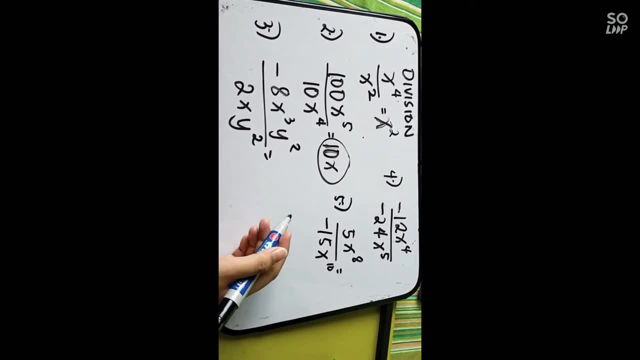 The answer is 10.. Copy the variable. We have here X, Then 5 minus 4.. The answer is 1.. So we have here 10x. Ok, 10x raised to 1.. So kahit wala naku raised to 1 yan. 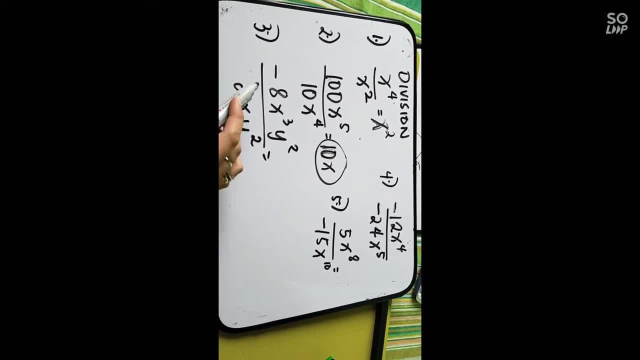 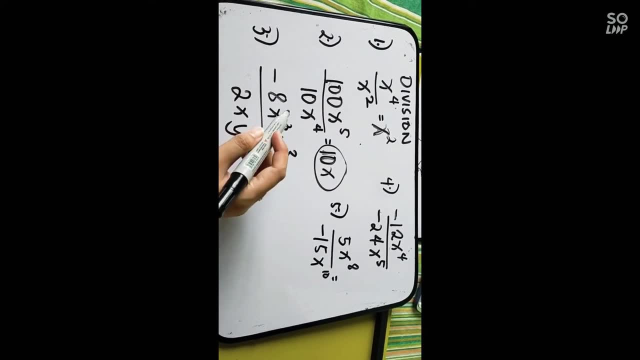 Okay, na po yan. Ok, Next tayo. Negative 8: x cubed y squared, Divided by 2x y squared. For this one, You are going to divide the numerical Negative 8.. x cubed Negative 8 divided by 2, the answer is negative 4.. 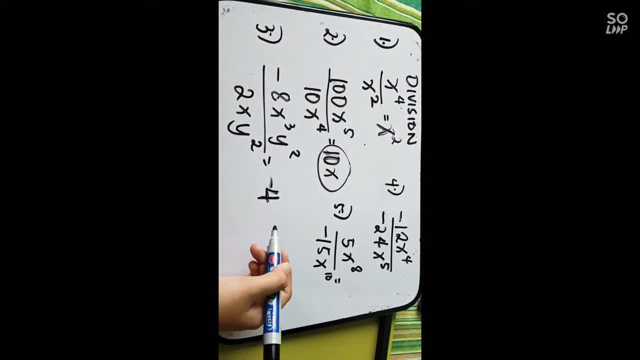 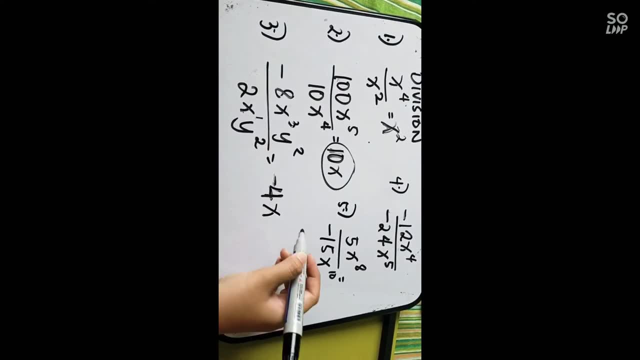 Negative 4.. Alright, negative, 4.. Then the variable copy X. So we have X cubed divided by X, This one is 1.. 3 minus 1, the answer is 2.. So we have X squared. 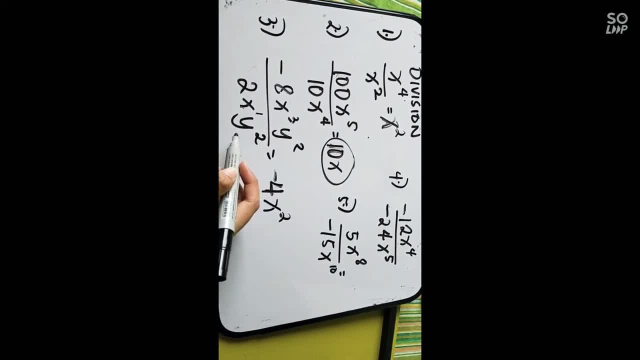 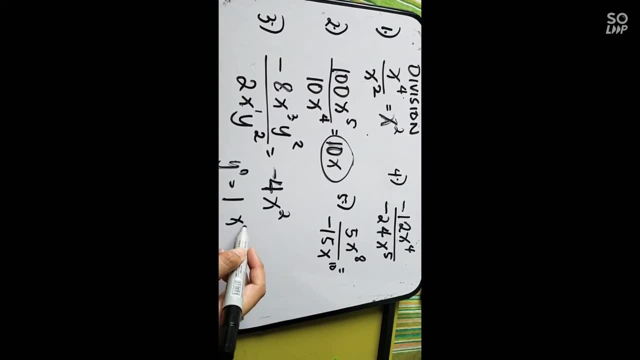 Then Y squared. divided by Y squared, the answer is Y raised to 0.. Any number that is raised to 0 is always equal to 1.. If X is raised to 0, it is always equal to 1.. So this one is cancelled out. 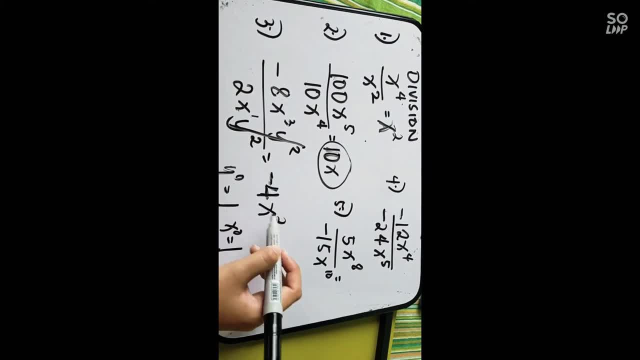 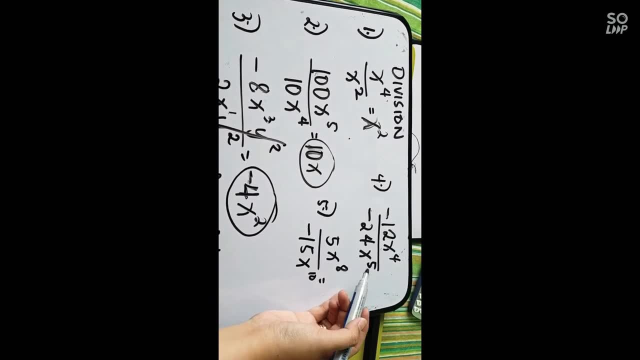 It will just be 1.. So 1 times negative 4, same for the answer. So the answer is negative 4 X squared. Is it clear? Then number 4, we have here. What do you notice? 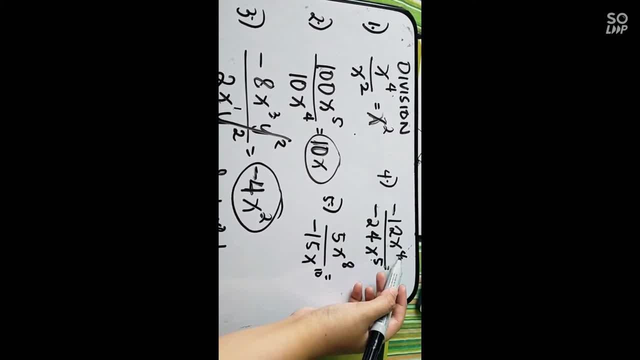 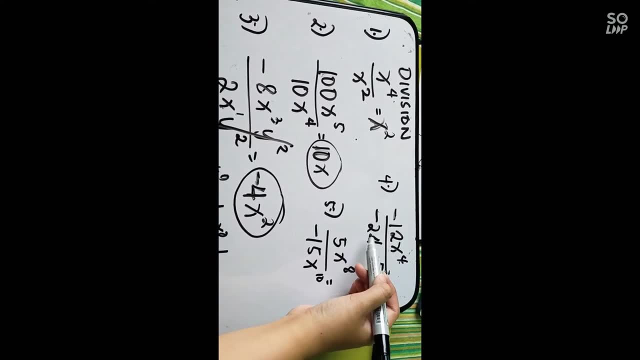 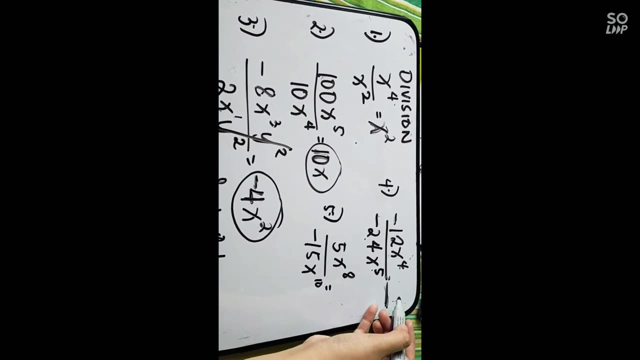 So the exponent of the denominator is bigger than the numerator. Okay, So for this one you are going. we have here negative 12 divided by negative 24.. So that is positive. So this one. it becomes divisible by 12.. 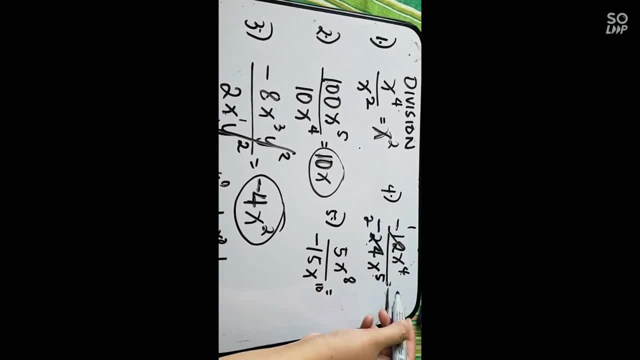 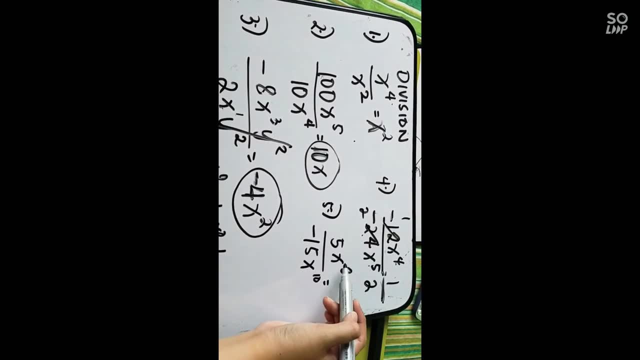 It will be positive. So this will be 1 and this will be 2.. So we have here 1 half, 1 half, Then the X, where the exponent is bigger, you will put it there. So, since the exponent of the denominator is bigger, you will put the X here. 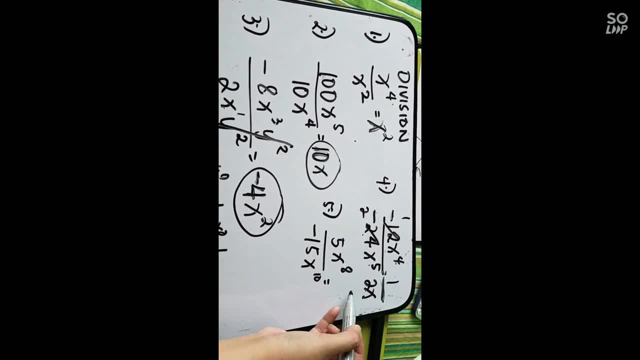 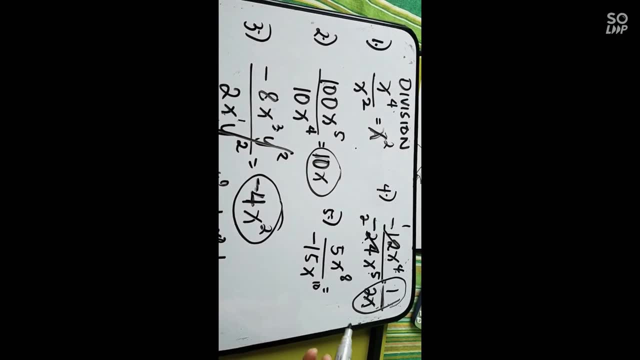 Now subtract So we have 5 minus 4.. The answer is 1.. So this one is the answer. No need to have right 1.. And then there is none. There can be some. Okay. Next we have here: 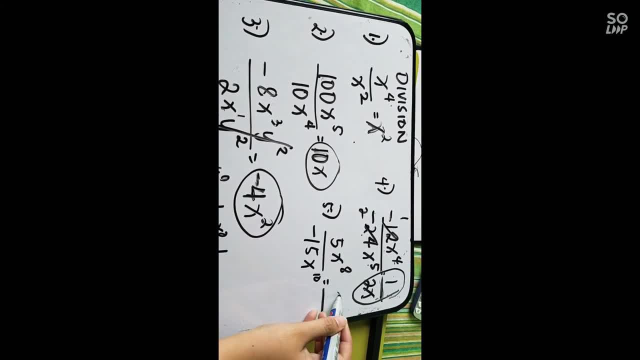 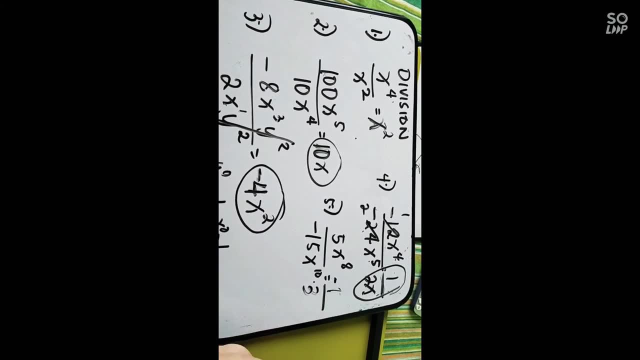 5 over negative 15.. So 1 is still here, Then this will be 3.. So the negative: you can put it at the top or at the middle. Okay, So then, as you can see, it is higher again. 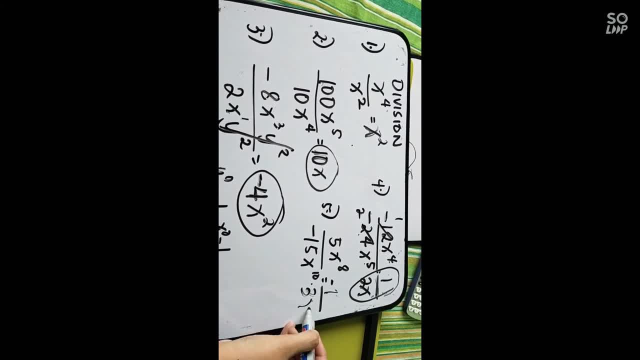 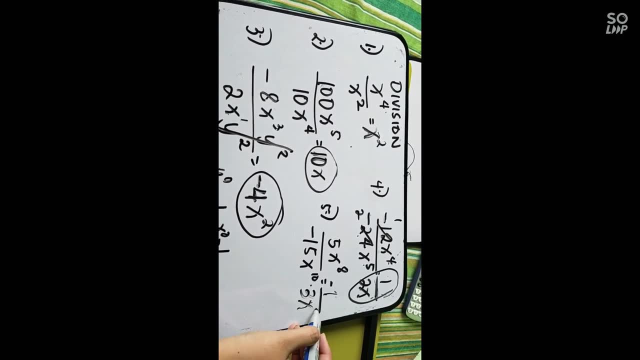 We have here X. The denominator is higher, so we will put it at the side of 3.. So we have here 3X. Then subtract 10 minus 8.. The answer is 2.. So the answer is 1 over 3X squared. 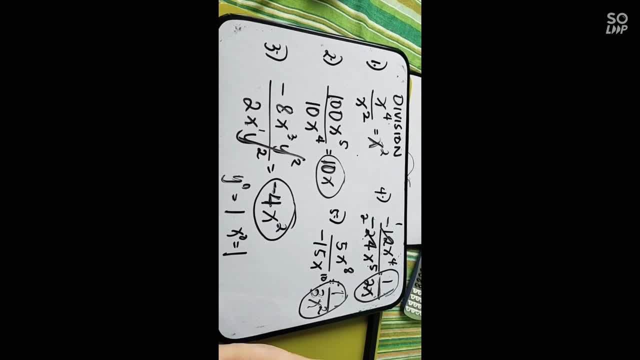 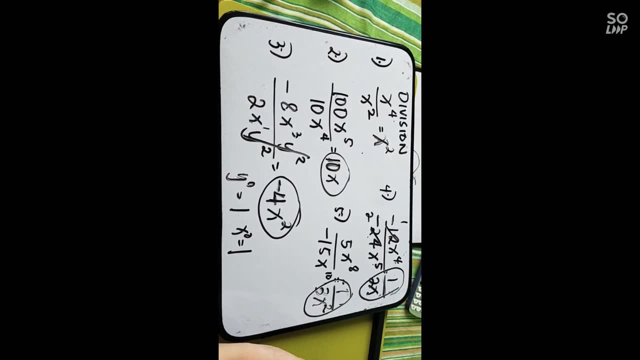 Is it clear? So that is the version. You are going to copy the variable, then subtract the exponent. As for the numerical coefficient, you are going to divide the numerical coefficient. Is it clear?